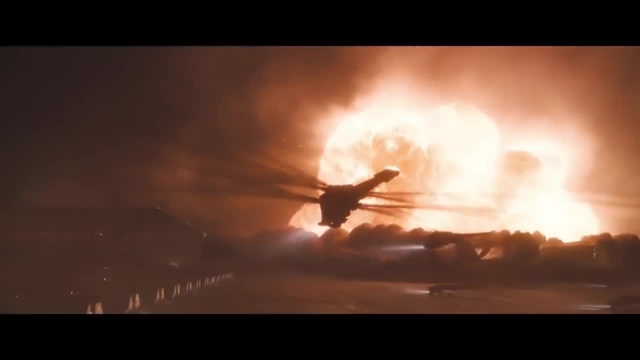 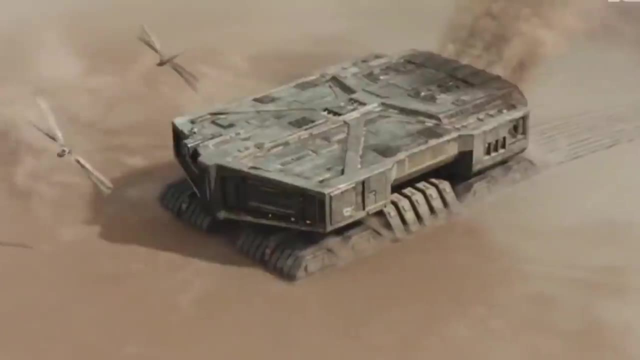 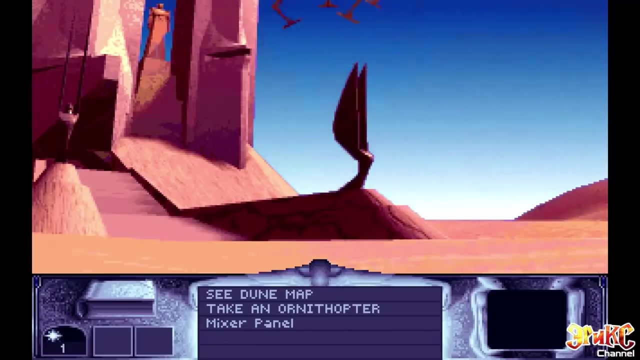 what flapping insects use. All in all, the Imperium thopters are fascinating machines that can use different modes of flying to their advantage. This machine has captivated people's fascination not just from the movies, but also from the computer games that came out in the 90s. However, when looked at from a practicality point of view, the thopters would 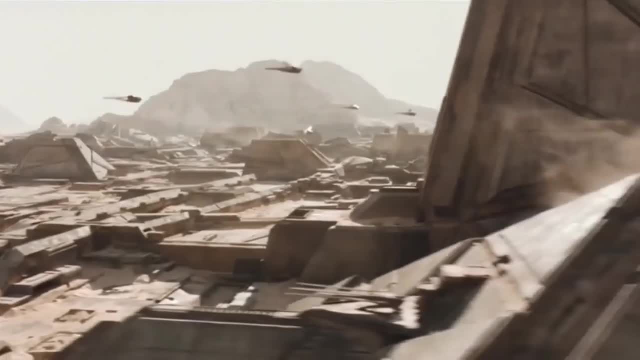 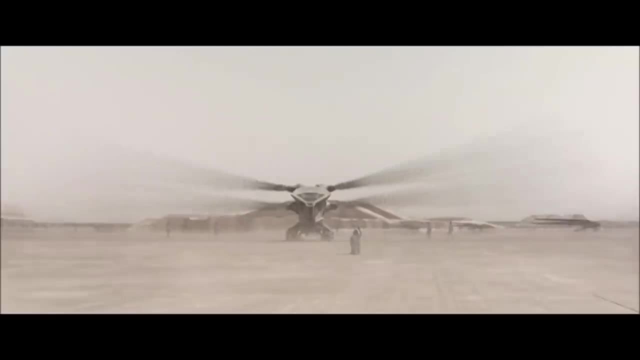 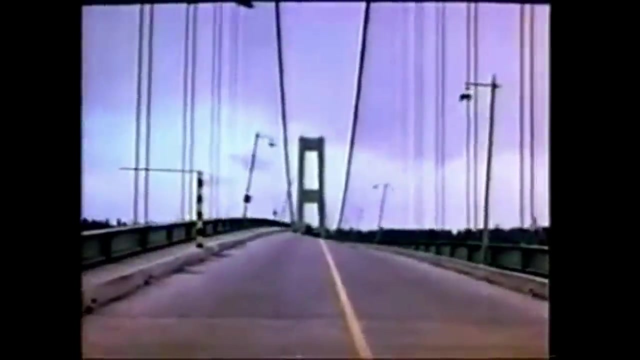 not be functional, especially the way they are shown to work in the movie. This is due to two main reasons. One of them is the extremely high frequency of vibration of the aircraft wings. Any structural engineer would tell you that high frequency vibration is structurally damaging. 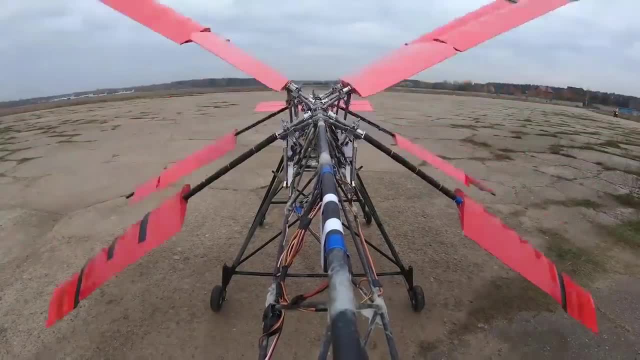 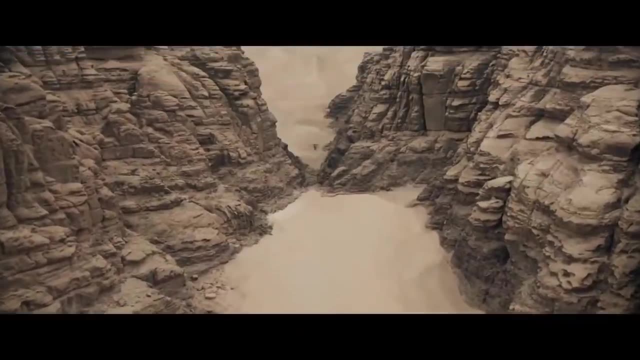 and is difficult to isolate. This means that even if we somehow find a wing material that is robust enough to withstand the high level of vibration as shown in the movie, it would be difficult to isolate the rest of the airframe, the components and its occupants from the vibration. 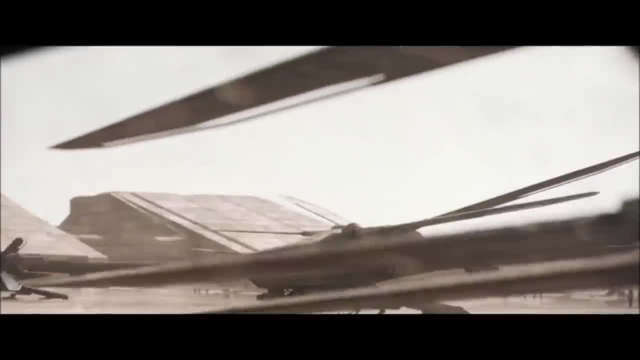 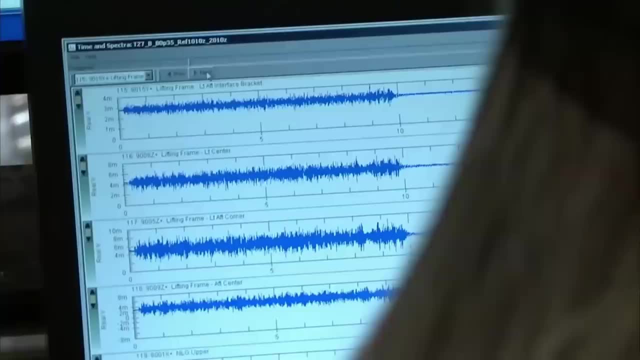 The wings are cantilevered to the mainframe, which means that the vibration-producing component is present inside the airframe. For structural integrity, the aircraft are designed to minimize vibration. In fact, there are systems being designed that now seek to harness the energy from the process. 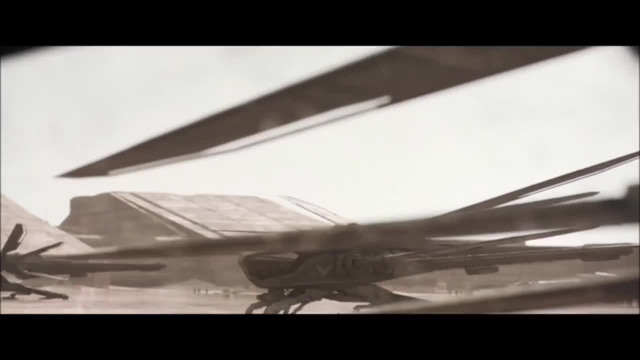 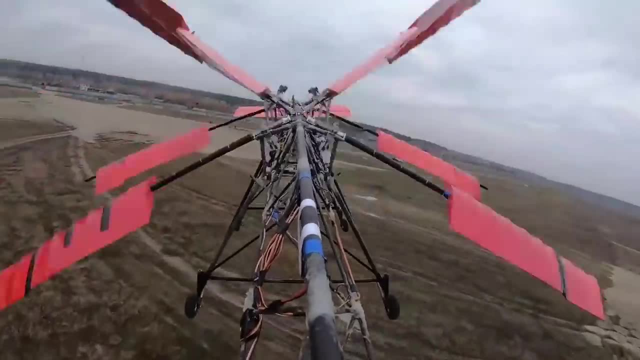 of vibration damping in aircraft. The second reason is the nature of the flap, particularly when taking into account the scale of the aircraft. The flapping wing in an ornithopter has to change its angle of attack during the upstroke and downstroke. This requires a much 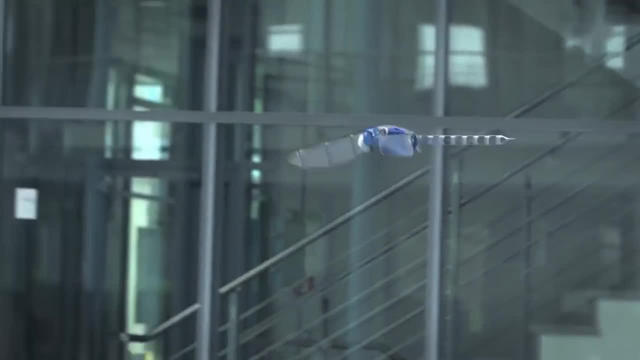 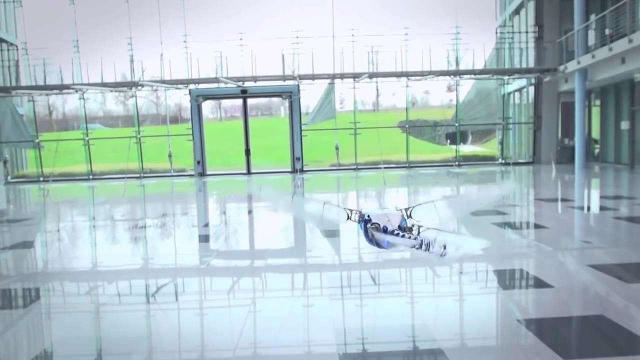 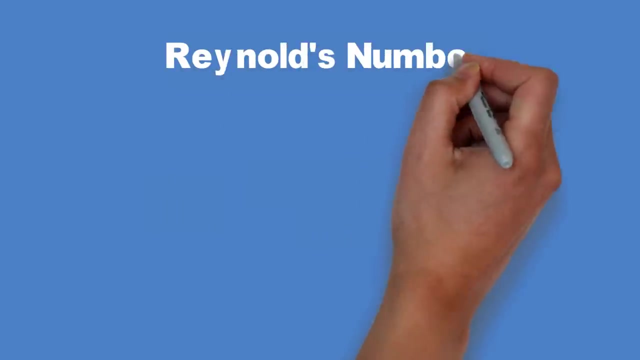 more complicated mechanism. No net lift would be produced in one particular direction if the wing simply waves up or down without changing its angle, Or in other words, the wing profile needs to change its orientation as it cuts through the air. We have to grasp an important fluid. 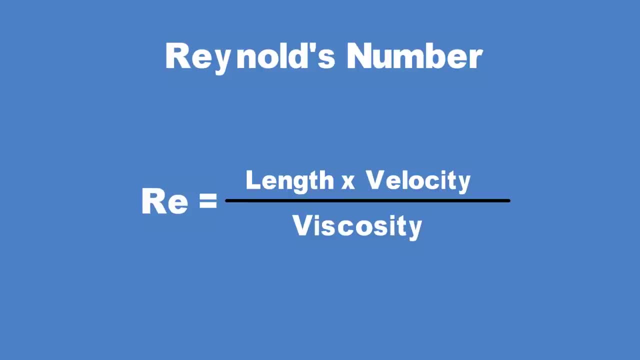 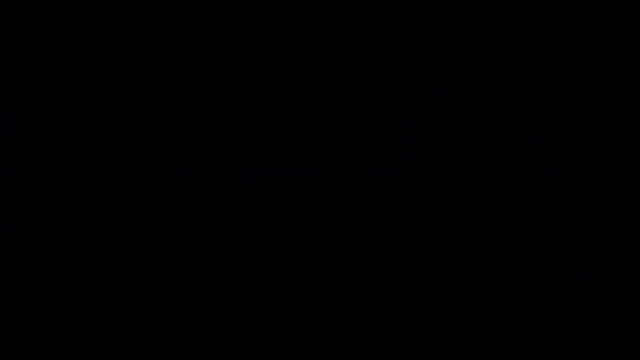 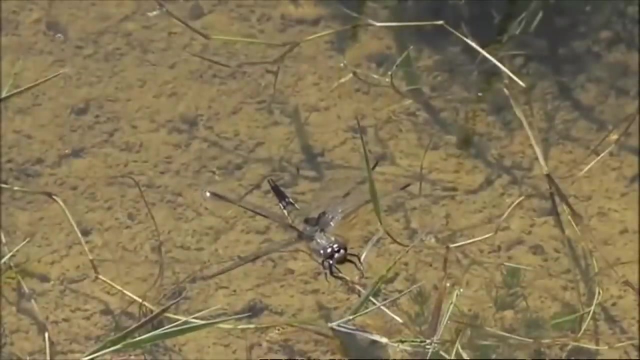 mechanics concept that is called the Reynolds number. In short, it is the measure of thinness or non-stickiness of the fluid in reference to the object of study. One can understand that an insect trying to flap its wing in a fluid-like water would find it difficult to do so. 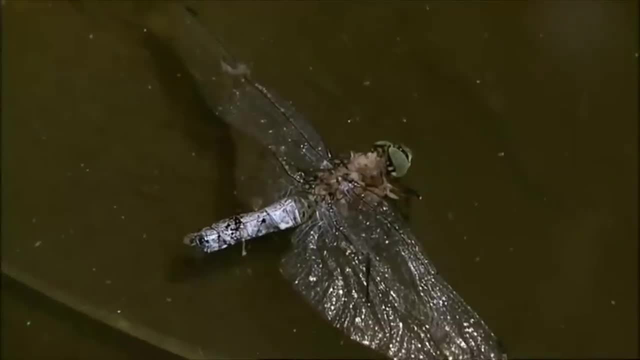 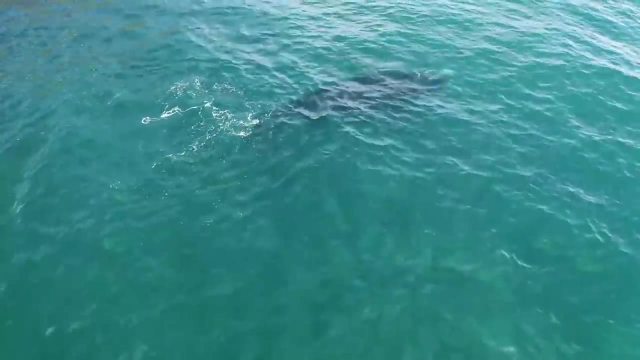 In some cases it would not be able to move its wing. even slightly Larger animals like a whale, on the other hand, would be able to move through the water without much difficulty. So for the whale, the water has a very thin and non-sticky feel, while for the 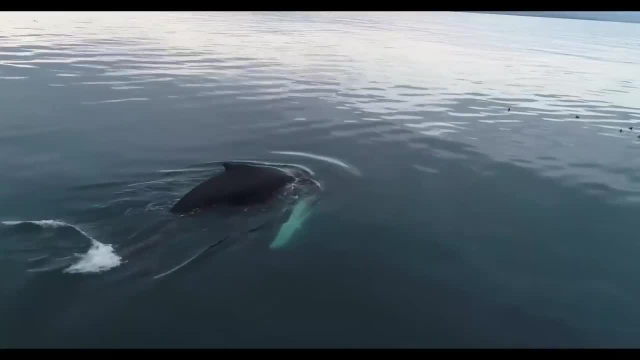 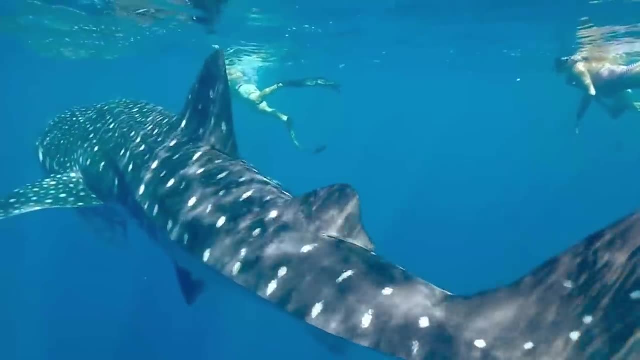 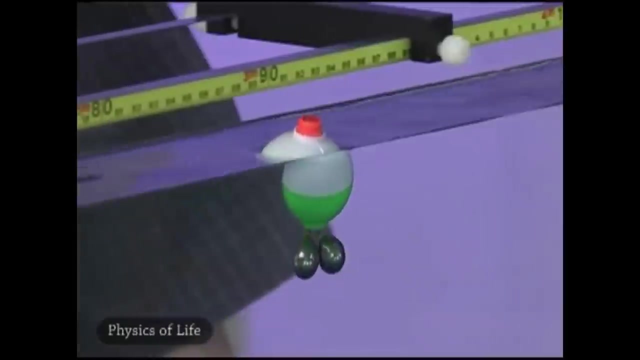 insect. it is the opposite, Even though it is the same fluid, that is, water. the only thing that is different is the scale, and it is this measure of the relative stickiness that is called the Reynolds number. So if the viscosity of the fluid is high and the scale of the 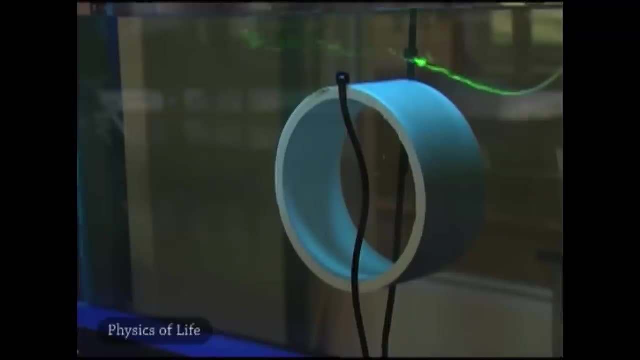 object is small, then the Reynolds number is low. On the other hand, if the viscosity of the fluid is low and the scale of the object is big, then the Reynolds number is much higher. This means that the higher the Reynolds number, the effect of viscosity of the fluid is less. 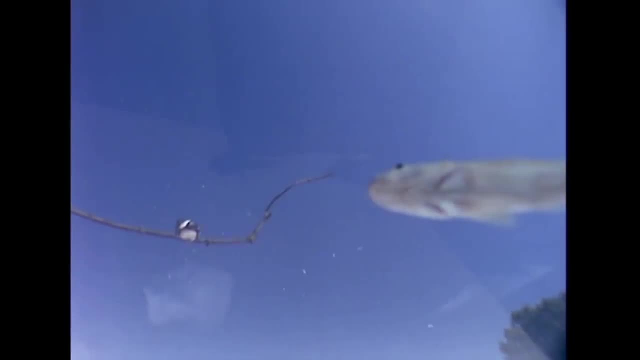 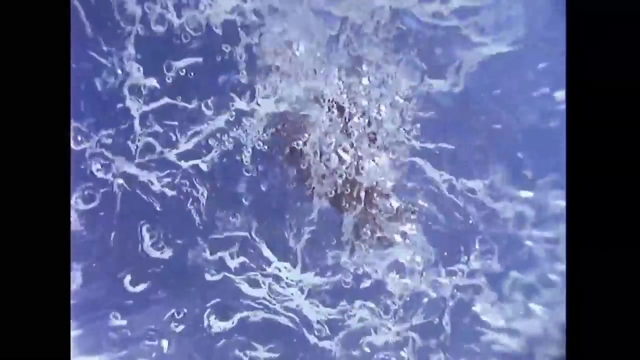 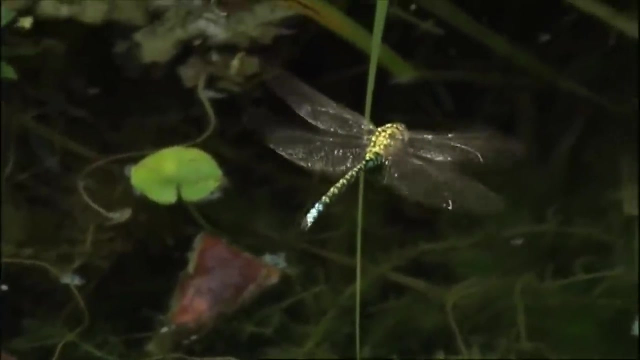 palpable on an object. Another factor that comes into play here is the speed of the wing movement. Again, the higher the speed of the object moving through the fluid or of its wing bead, the higher the Reynolds number. To unpack this concept further, imagine the dragonfly. 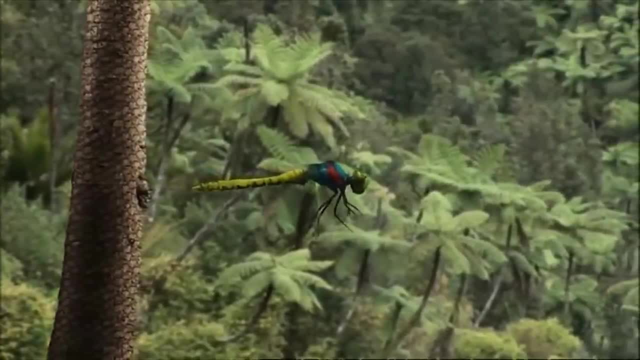 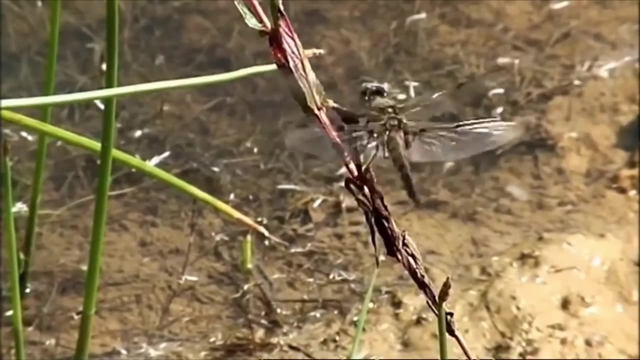 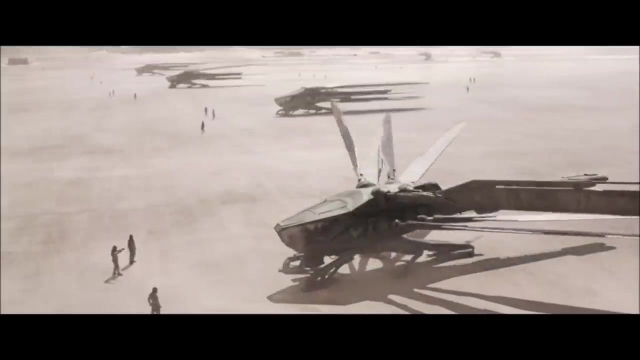 Now we can understand that to manipulate the air by means of wings is much easier for the dragonfly and is very controlled. This is because the fluid, as perceived by the dragonfly, is much thicker. When you now look at the Ornithopter scale, air is the same, but the scale is bigger. Therefore, 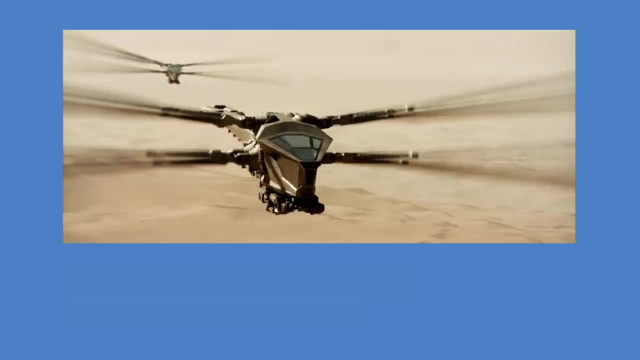 to mimic the same flying conditions as the dragonfly. the frequency of the wing bead of the Ornithopter should not be higher but lower than the dragonfly. It should be the same order of magnitude. lower as the scale is higher. Only then the 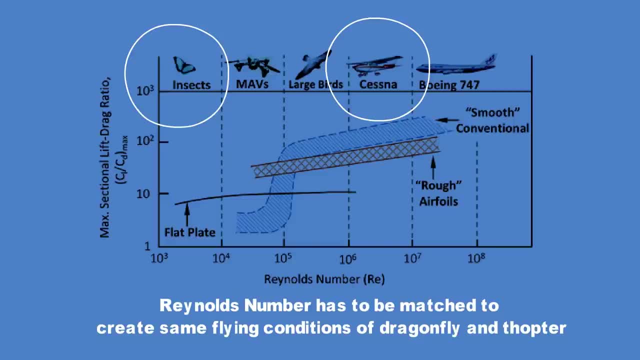 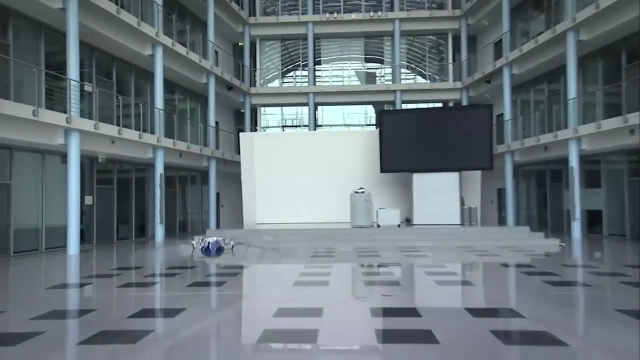 aircraft will match the conditions that are similar to dragonfly and damselflies. It is much easier to create a vortex at a higher scale than it is at a smaller scale. The leading edge vortex that is generated by the four wings of the dragonfly is anticipated by the 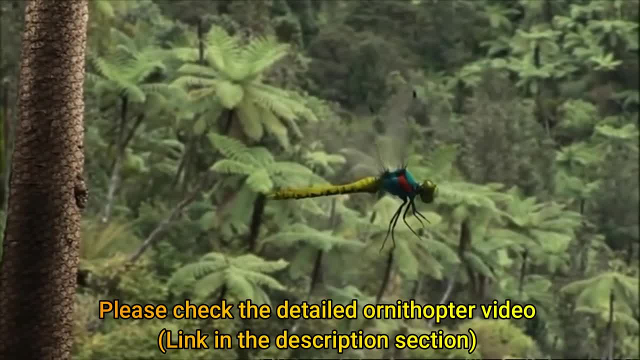 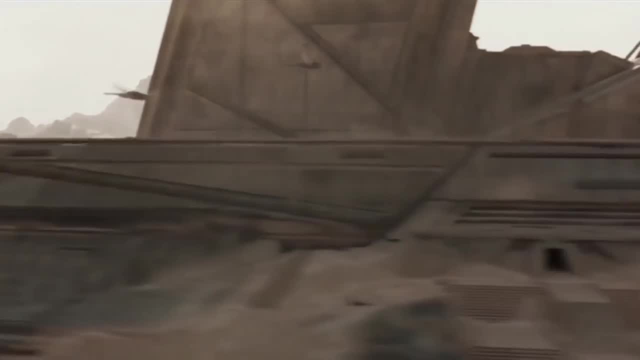 hind wings, and the energy imparted on the air by the four wing is collected by the hind wing. So while the Ornithopters can be produced, it should be done with a lower wing bead but with a higher stretch. This will also be beneficial from a vibration isolation. 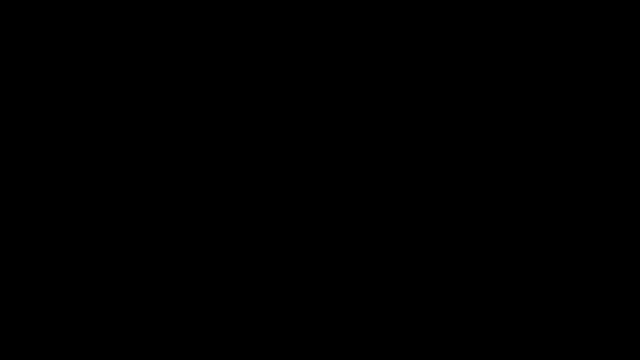 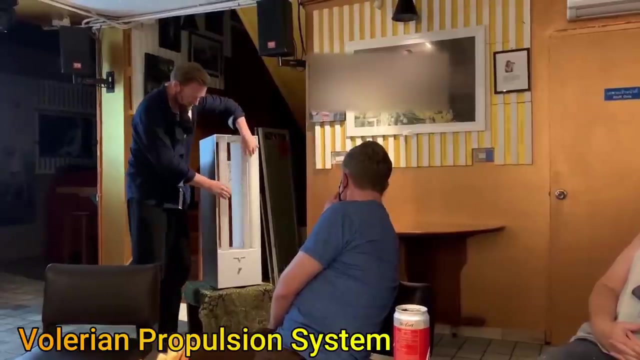 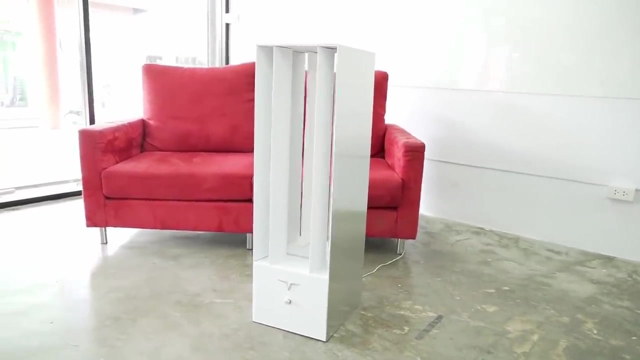 and structural integrity point of view. Having covered the thopters, let's now look at a very interesting system that has been termed as the Wallerian propulsion system by its inventor, RIM. Can it create flapping wing aircraft of another kind? Let's find out. 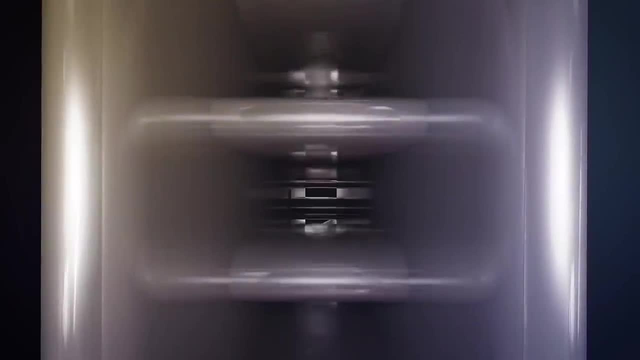 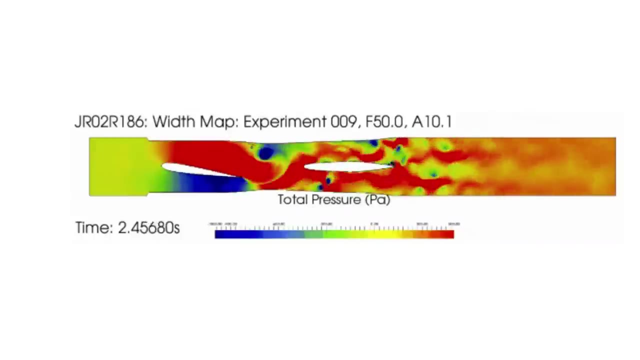 According to the inventor, the Wallerian fluid system consists of an internal airfoil that is present in a duct. It is driven by a cam on a rotating shaft, which allows the airfoil to do a waving motion. As a result, the air is pushed downstream where a static airfoil is present, and 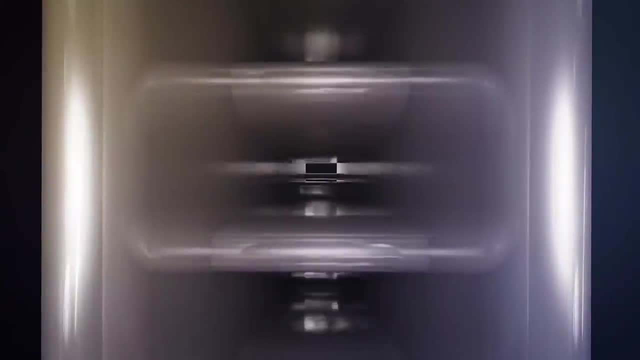 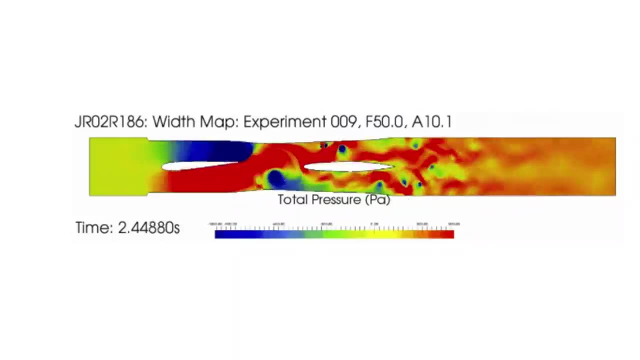 creates lift. The placement of the waving wing inside the duct increases the air flow. The air flow increases the pressure differences, which in turn enhances the flow rate. The waving duct wing creates a stream of thrust-producing vortices known as a reverse Karman vortex street. These 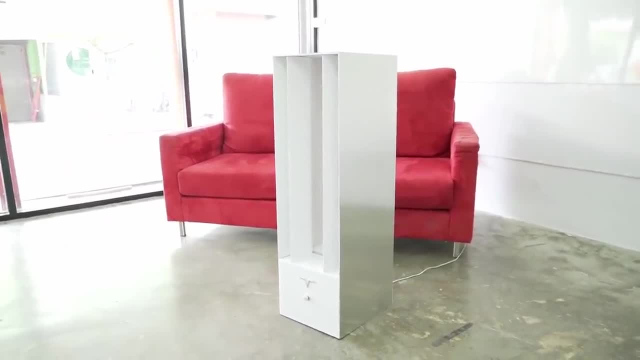 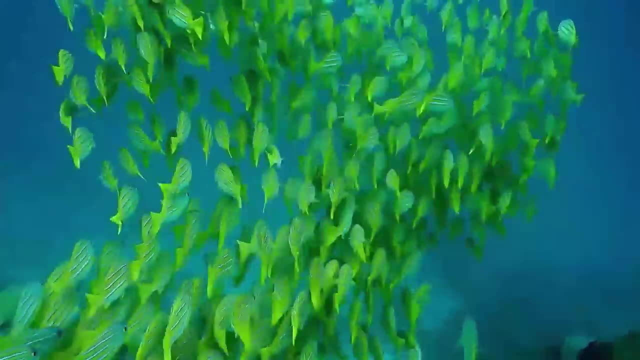 energy vortices are passed through a converging-diverging section and thereafter passed over a static airfoil. This system is based on the same principle as the movement of fish. Sets of these wing and duct units are typically placed together to form an array. 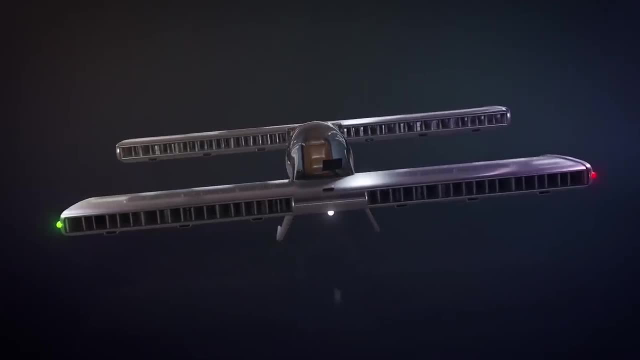 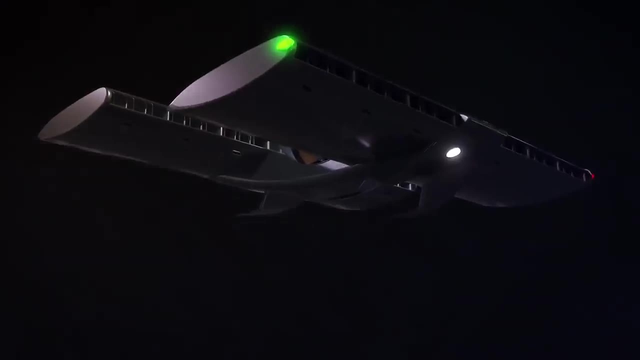 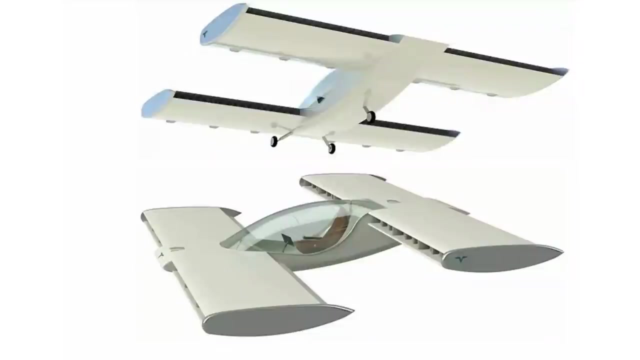 In many of the aircraft concepts, this array itself forms a wing leading to a highly integrated propulsion control and lifting structure. The claim by Wallerian is that this system is more efficient than a propeller. They have created several concept designs for different 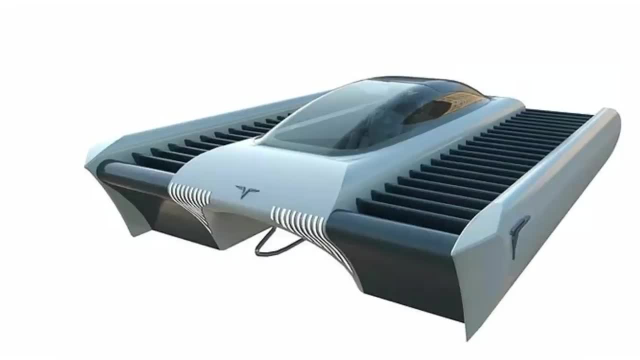 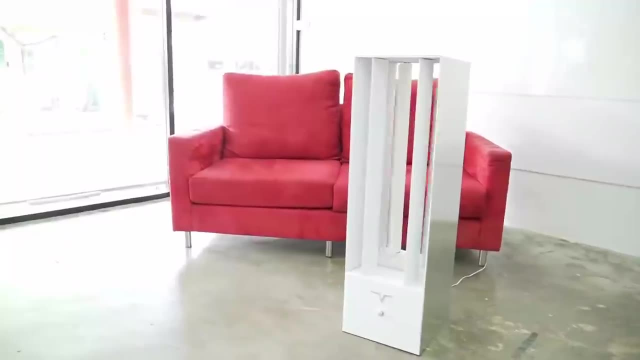 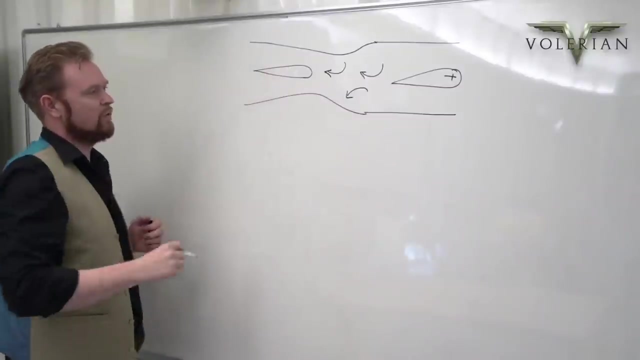 applications and missions. While the usage of the Wallerian propulsion system remains to be seen, even in a subscale model, they have produced a room fan based on the same technology, which they are claiming to be on sale soon: The Wallerian propulsion system. 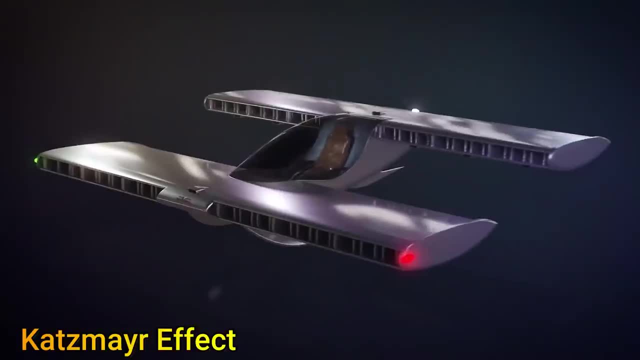 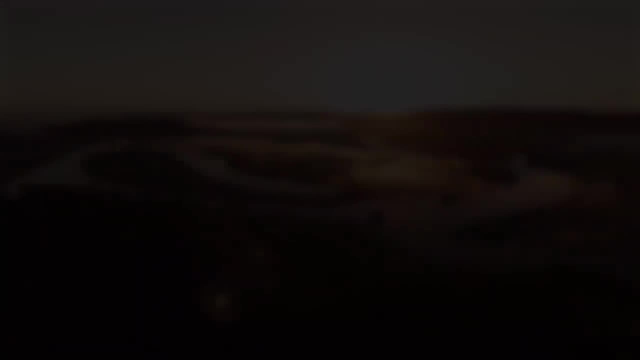 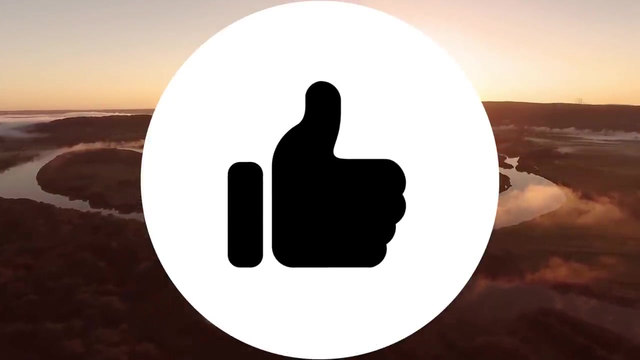 is based on a very little known Kastmeer effect. We will keep an eye on this technology and present a deep dive video on the concept in the future. And with this the video is concluded. If you learned something from it, please do give it a thumbs up. Thank you for your attention.